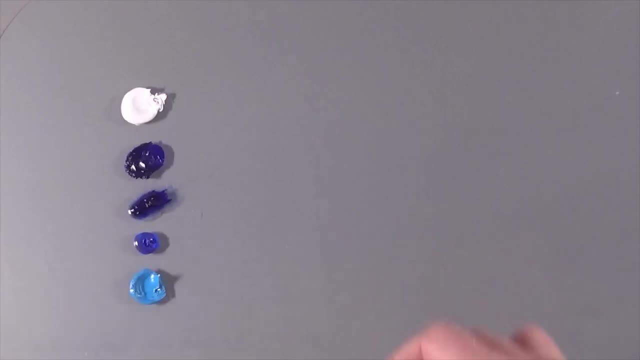 more violet hues at the top, down to the very pale colour at the skyline at the horizon. sorry, Okay. so if I just take a little bit of these and lay them out, you can see that these top two are very, very transparent colours. 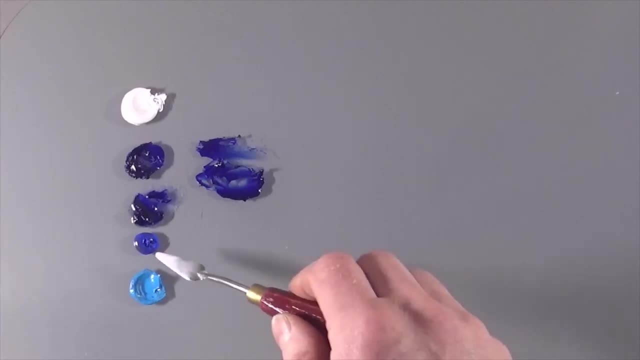 So that's the ultramarines, And then below that we have cobalt blue, which is a nice translucent colour, And we have the cerulean at the bottom, or cerulean, depending on how you want to pronounce it. If we just mix just a touch of white through those, you'll see that we can very quickly produce. 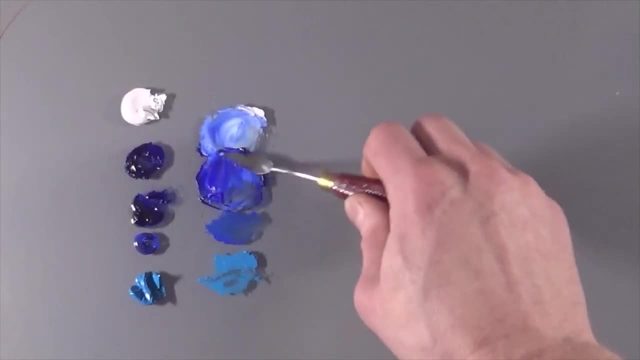 a really pigment-rich colour. So that's the very first version of what I'm about to do, just using ultramarine. Now, if you don't have these colours in your box- and that's quite likely, I suppose if you are just starting out- no issue with that whatsoever. Many ways to scan the cat. 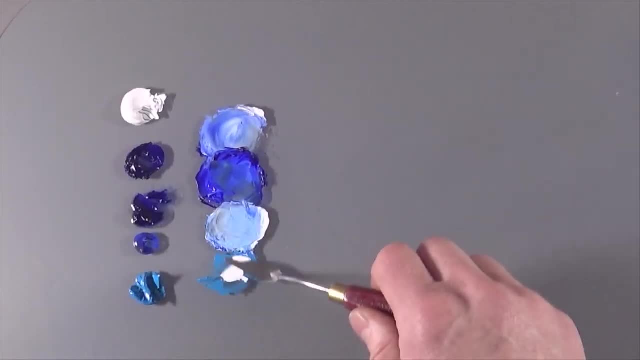 So what we're going to do here is we're going to look at the other way to get these same colours. Okay, so there we go. There's the sky As it progresses down. mix a bit more of the cobalt blue in there. 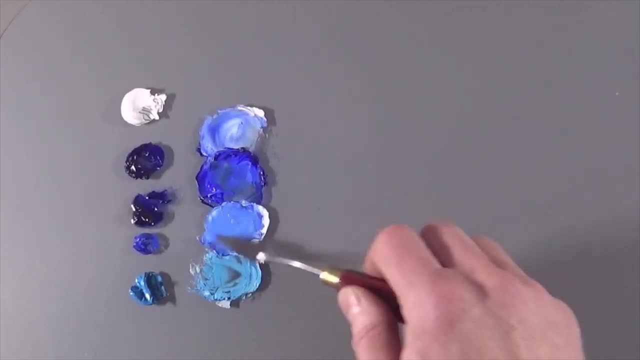 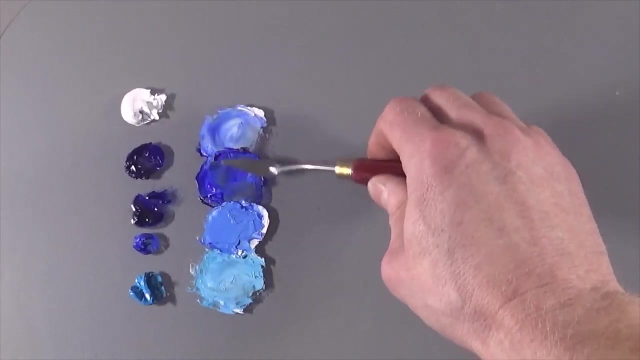 from the kind of the deeper, warmer tones at the top to the washed out horizon colour. So that's the sort of pure tubes version. Just blend them one to the next as you come on down the canvas. But what we can do- and you've seen this a fair few times now- 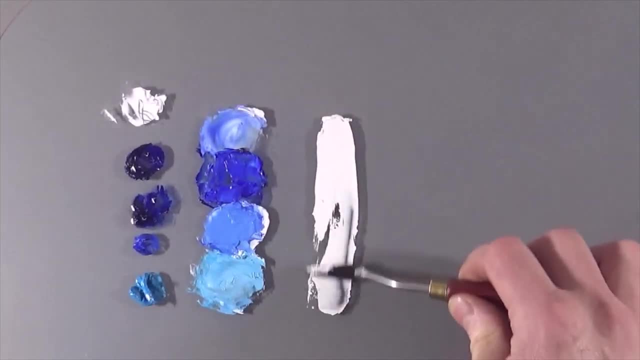 is, we can create a colour gradient and then take from that the swatches that we need. I'm just going to switch over to a different palette knife here, So what I'm going to do is I'm going to take a pile of the ultramarine blue here. 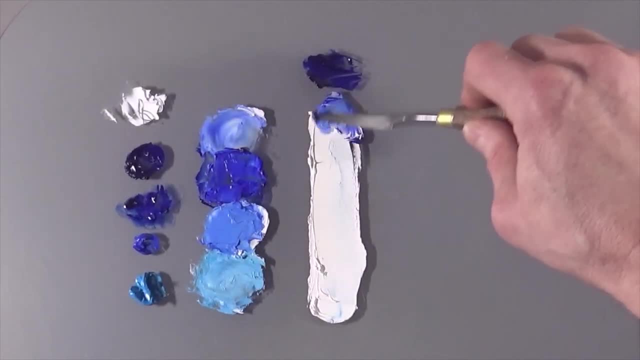 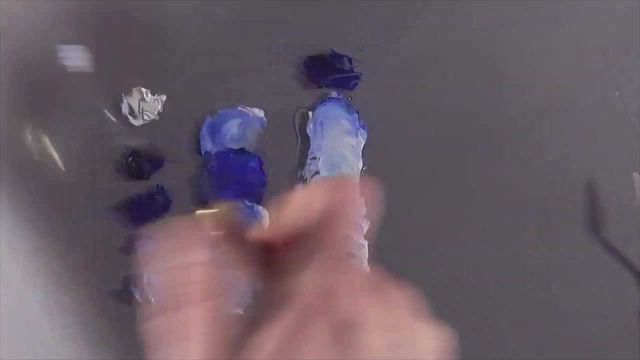 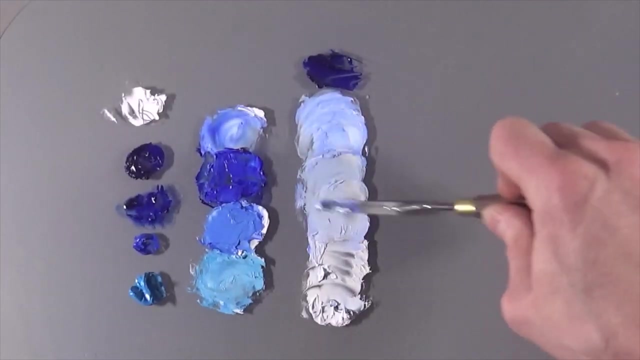 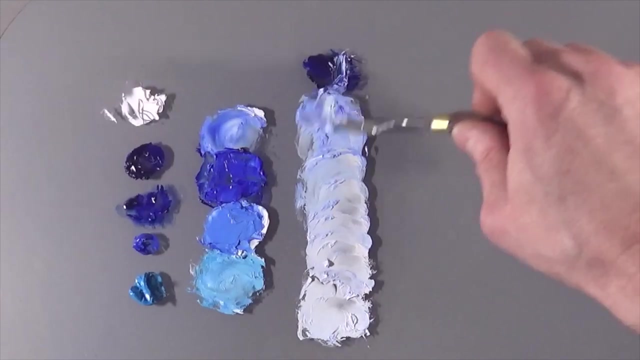 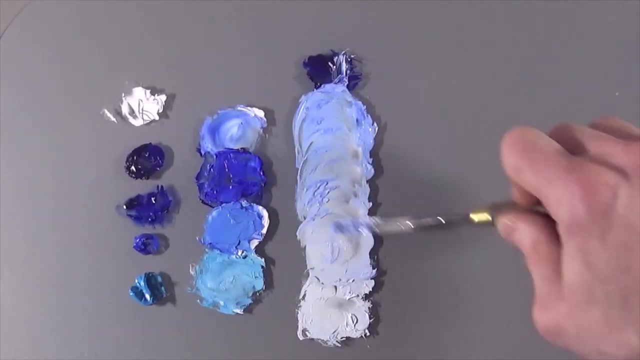 I'm going to put all of this through. It's a very, very thin layer of colour intense pigment and I'm basically just going to work that away down. just drop a little oil into this as well. bring a little bit more of that blue through. 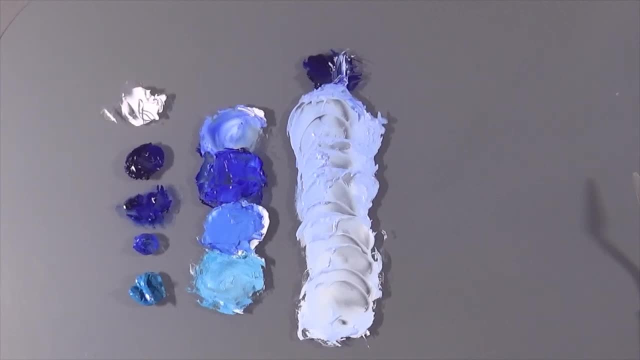 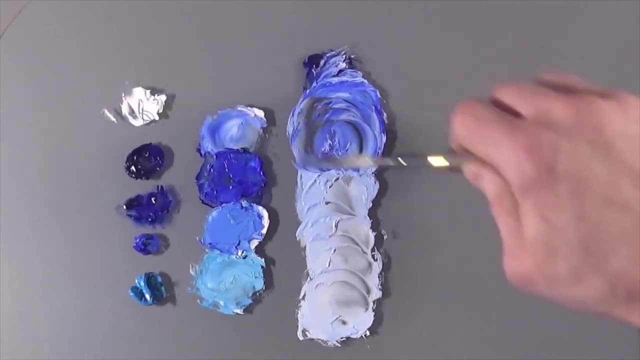 intensity of colors that you want. it's intensity of colors that you want. it's the same mix all the way down ultra, the same mix all the way down, ultra. the same mix all the way down, ultra. marine blue, which is a very, a very marine blue, which is a very, a very. 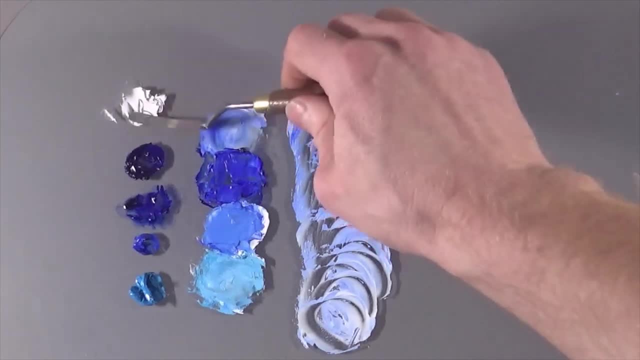 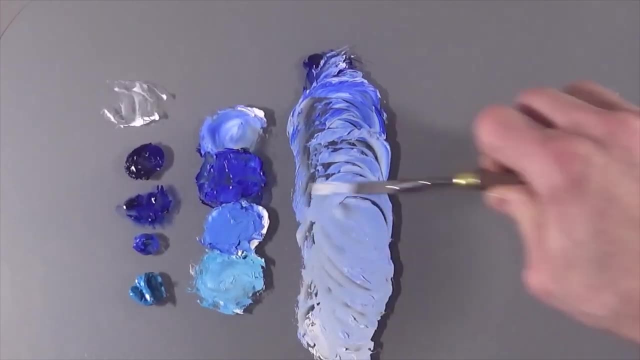 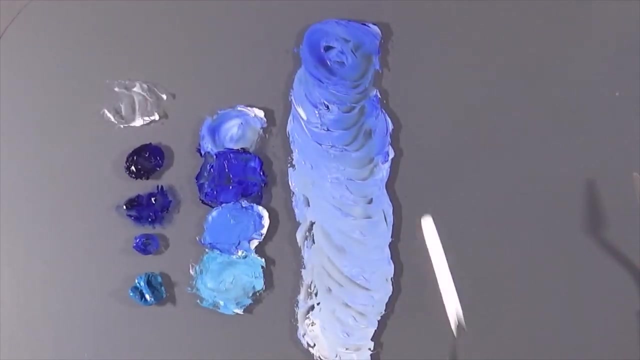 marine blue, which is a very, a very common color to to get in starter sets. common color to to get in starter sets. common color to to get in starter sets- very, very versatile color, basically very, very versatile color, basically very, very versatile color, basically going up to the lovely deep colors in the top. What we can do here with that now. 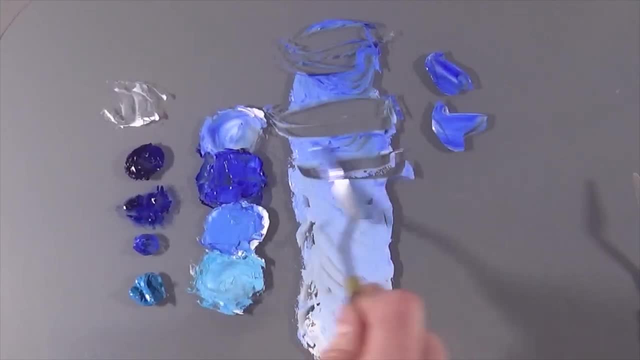 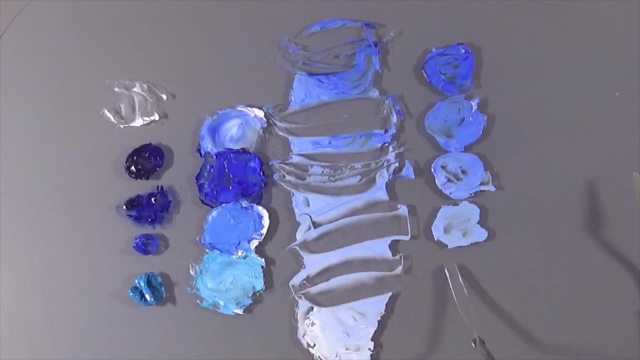 is pull out some representative color samples. It's often easier to see them in this form. There we go, so top of the sky, right the way down, As you can see here, not a million miles off. these colors- Cerulean blue- can sometimes need a touch of orange in to stop.